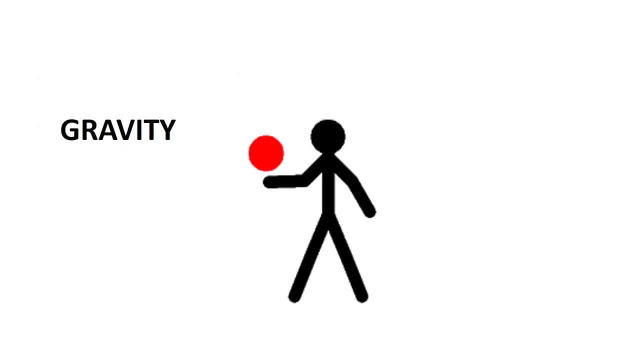 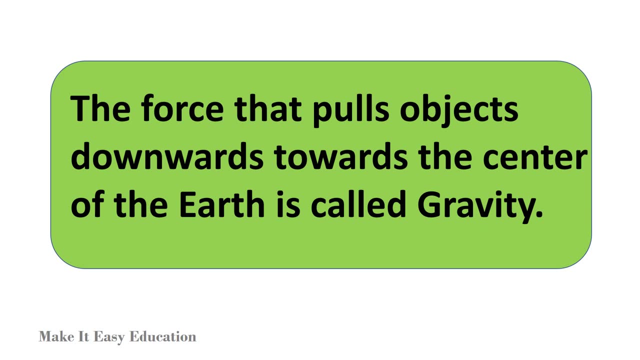 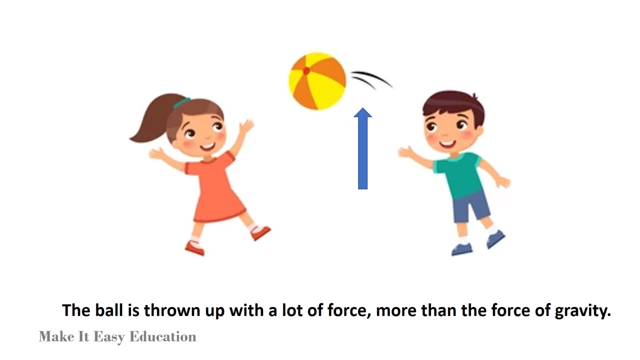 fall down. Why doesn't it keep going upward? This is because of the force of gravity. The force that pulls objects down Towards the center of the earth is called gravity. When you throw a ball up, you throw it with a lot of force that is more than the force of gravity, So it rises. As the ball moves up, it loses this. 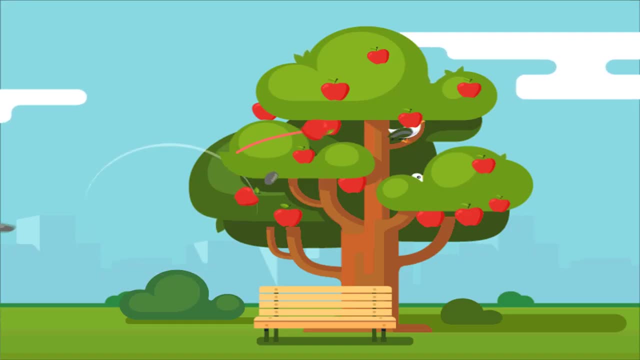 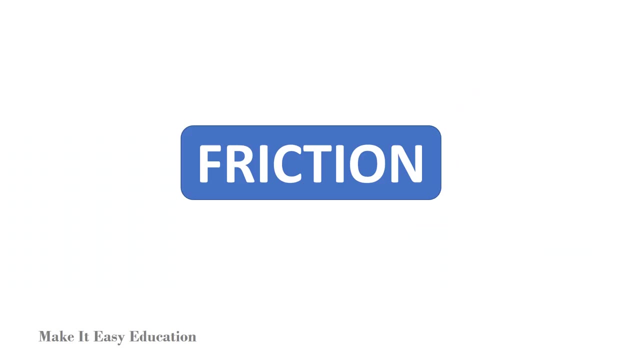 force and then gravity pulls it down. Similarly, leaves and ripe fruits always fall down to the ground due to the force of gravity Friction. When a ruler is pushed across a table, it stops after moving a certain distance. It stops because of friction. 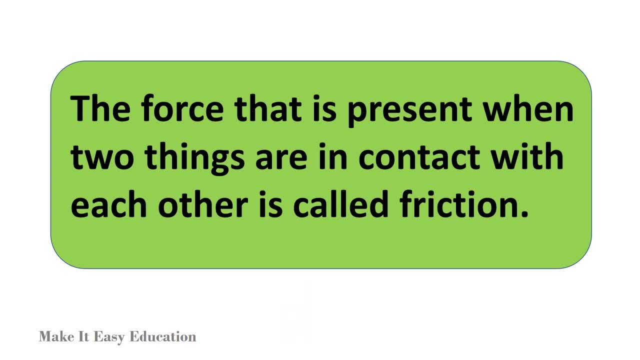 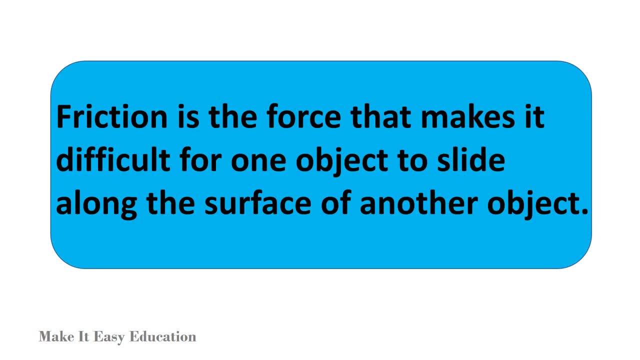 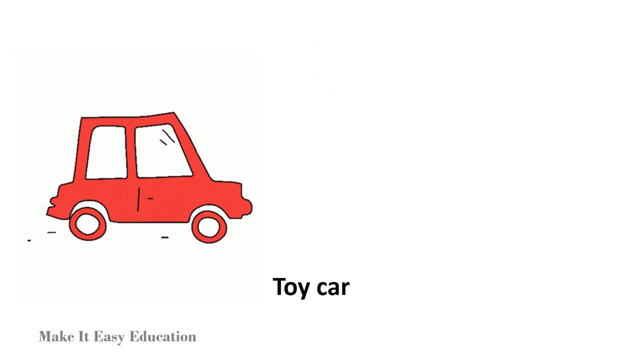 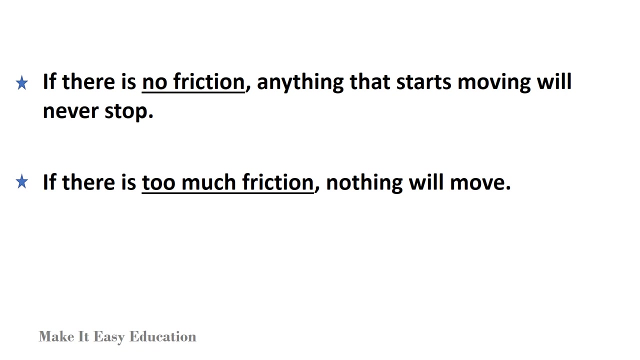 The force that is present when two things are in contact with each other is called friction. Friction is the force that makes it difficult for one object to slide along the surface of another object. Friction resists the motion of the object on the surface. As a result, the object either slows down or stops moving. If there is no friction, anything that starts moving will never stop. If there is too much friction, nothing will move. In fact, if there is too much friction, nothing will move. 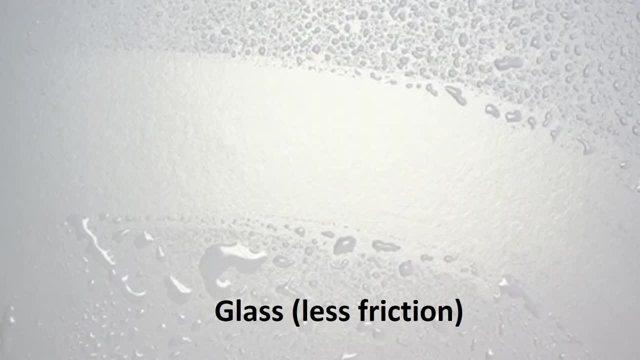 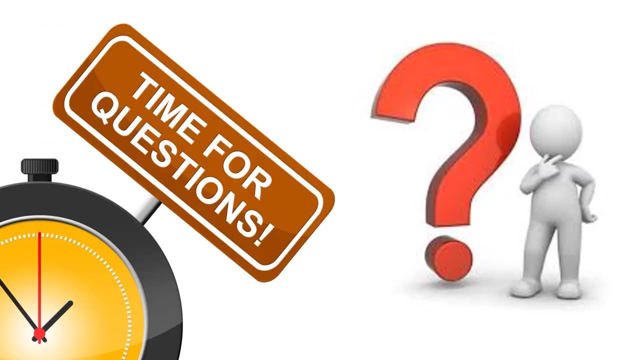 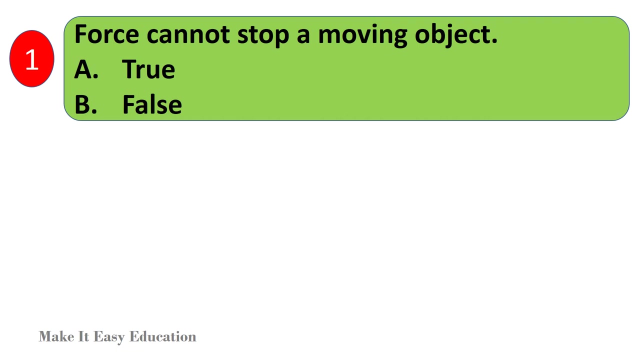 In general, materials with a smooth surface like ice or glass cause less friction than materials with rough surface like carpets. Question time During graduation: did you have travel problems? Yes, My dad didn't lied to me at school. 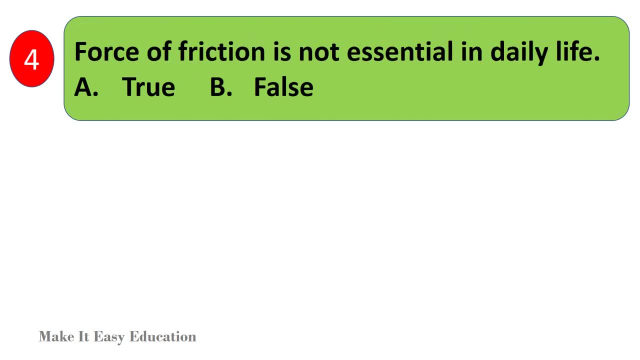 We eggs were supposed to be put underQu glass of water when we got to school. Cris is a town guy, which means it is not easy to put water in the water. Should U have traveled once? Dios mio, call my mom. 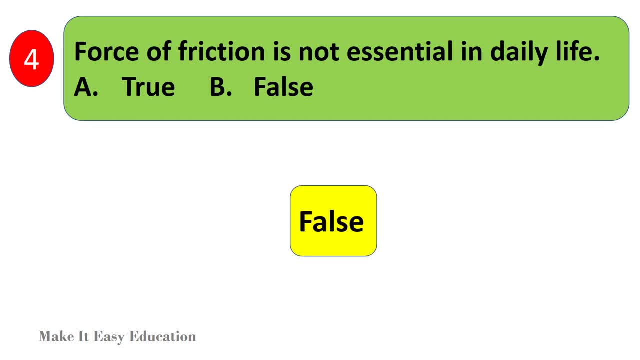 I want to be born again, But 다시 había que vegetar, pero Uarmara ya llenara el inflammado para que pudiera NXTE. Un día sabía la costa queить vida en la iglesia pantonta. Estaba Highermente Second Younger Me iba a ir al 되 un traves porte. 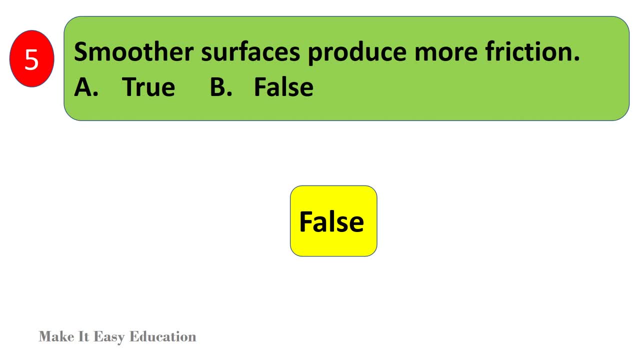 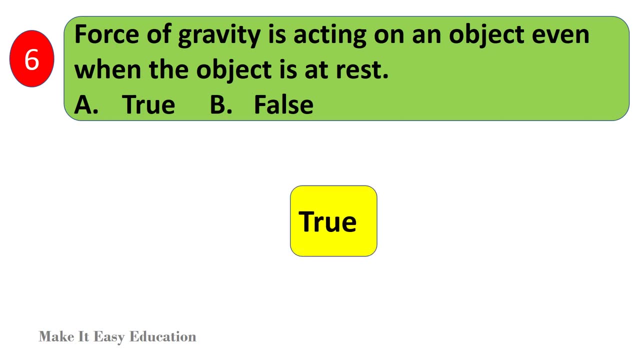 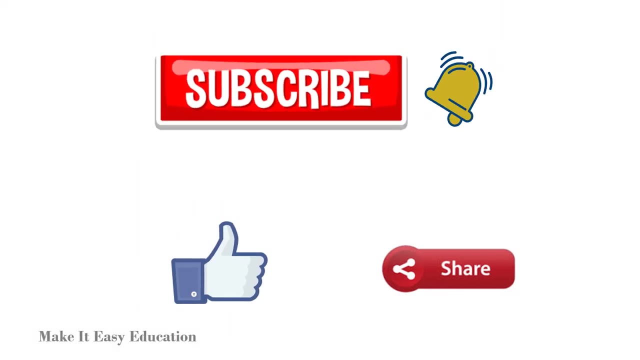 Conversely, de adentro, la suerte loin: acitan. No solía ждar fabrics, No, no, no Herbes, And also el regalo wardarme. every week you will be notified by a new video, so don't forget to subscribe and. 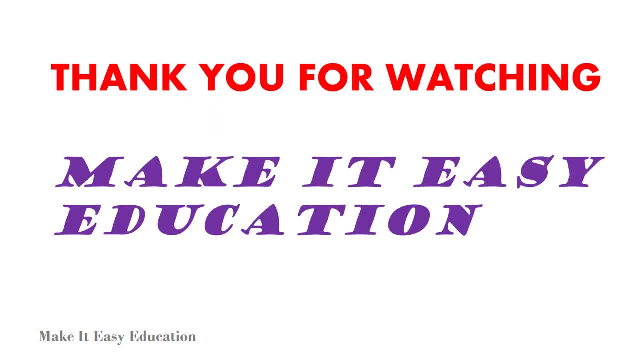 click the notification bell. thank you for watching. make it easy education.